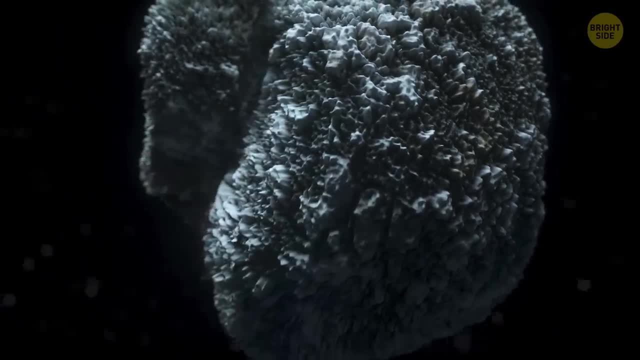 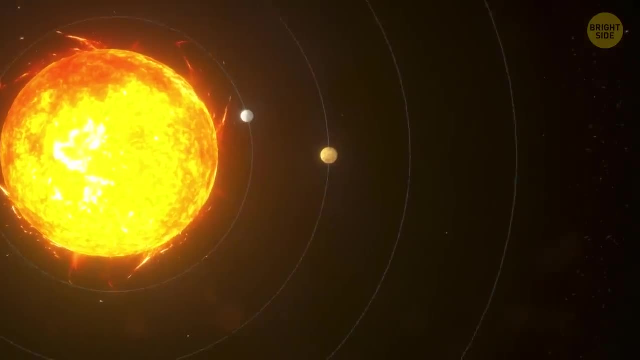 All eight planets of our solar system are unique and made of very different stuff. How about going on a space journey from the Sun to Neptune, the farthest planet of the solar system? We can check what's inside each celestial body on our way. 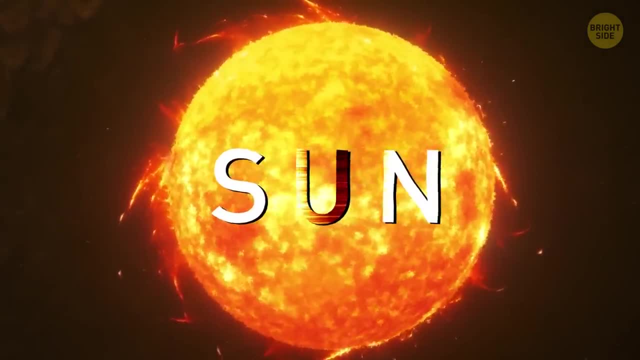 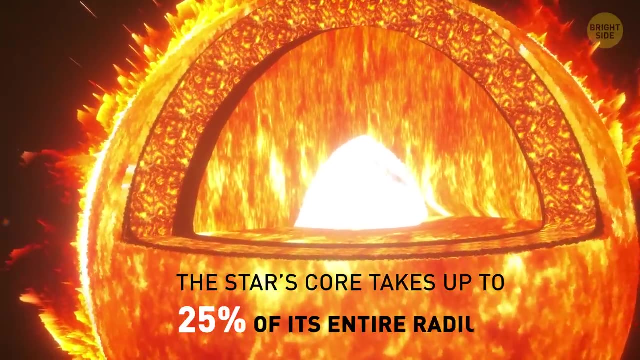 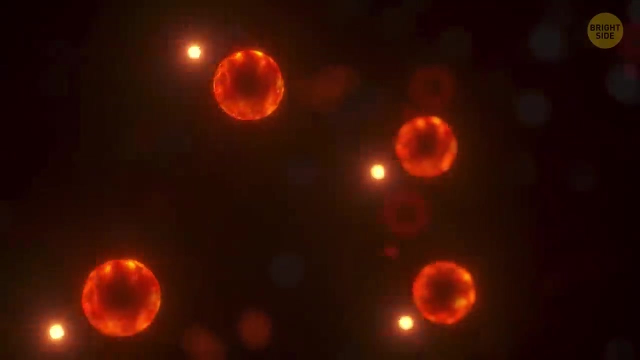 The Sun. We're starting our expedition from the Sun, a really big ball of gas and scorching plasma. The star's core takes up to 25% of its entire radius. Inside, gravitational forces create incredible temperatures and pressure which makes hydrogen fuse into helium. 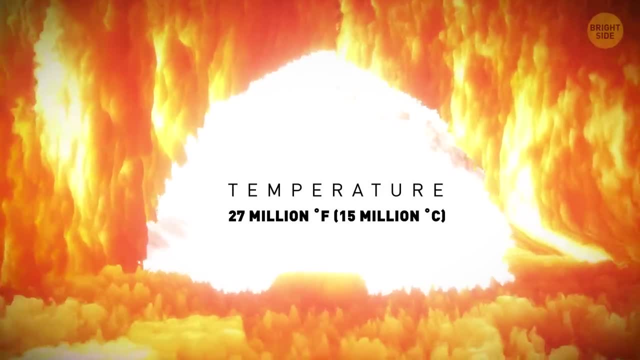 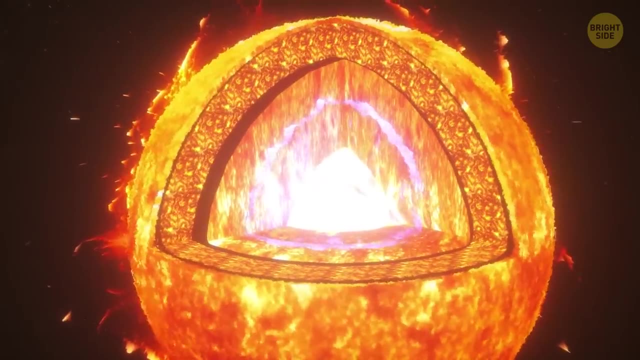 This layer has a temperature of 27 million degrees Fahrenheit. give or take All that energy moves to a zone called radiative. It takes, on average, 170,000 years for the energy to get all the way from the core to the next convective zone. 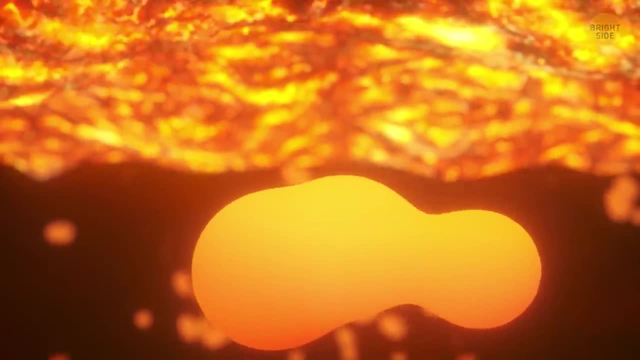 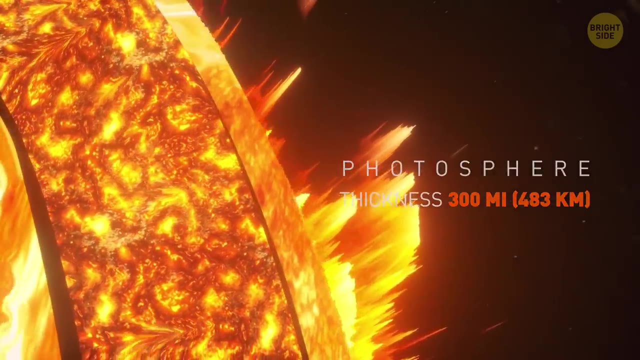 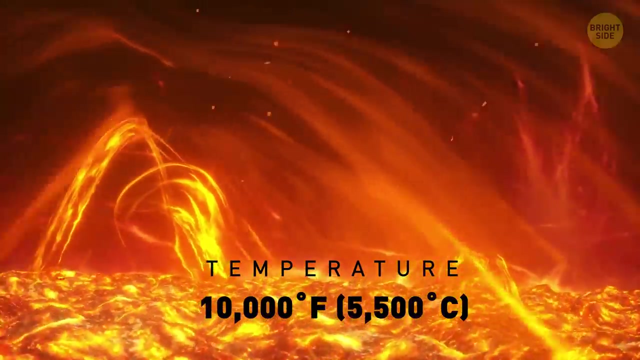 There, bubbles of hot plasma float upward And end up at the Sun's surface. That's where a visible 300 mile thick layer starts. This gassy zone- and don't I know about gas- is called the photosphere. It gets heated to 10,000 degrees and consists of granules, cells of plasma. 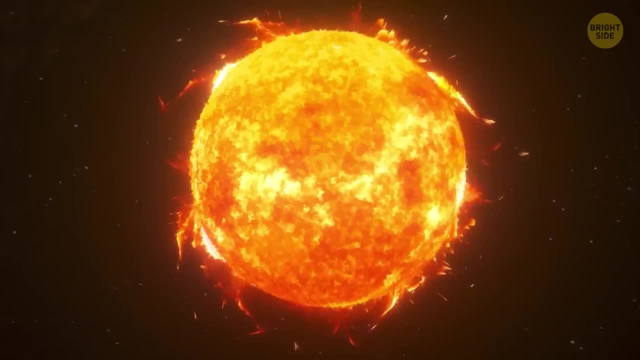 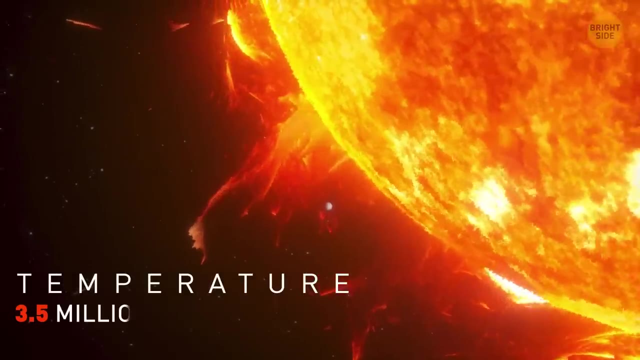 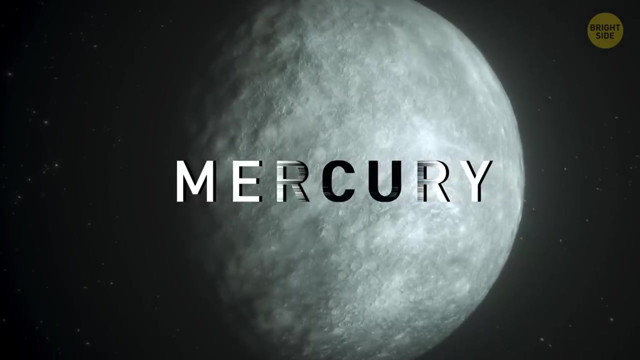 600 miles in diameter. each Moving further we get to the crown. That's the star's thin atmosphere. It's getting hotter again, with temperatures reaching three and a half million degrees, So we'd better not linger. Mercury: That's the first planet on our way. 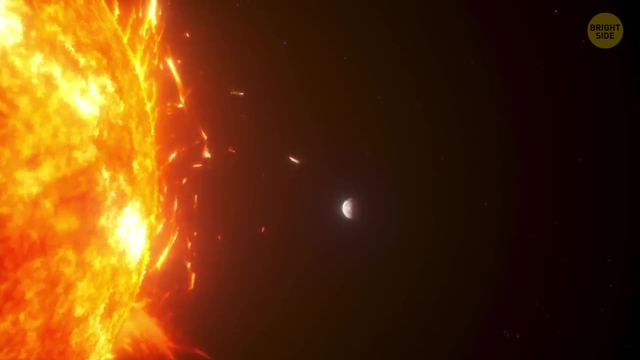 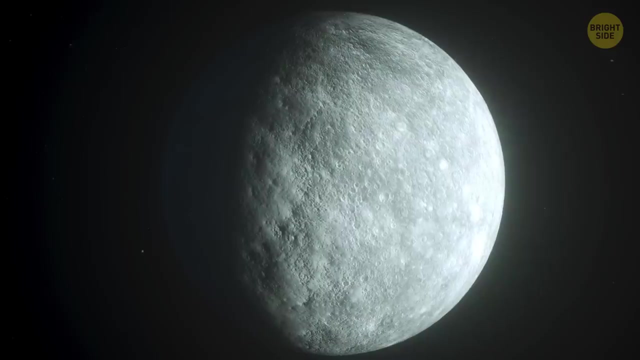 The smallest of all the four inner planets, Mercury is just 3,000 miles at the equator. It's also the second-densest planet, topped only by Earth. Mercury has a massive metallic core. It takes up almost 85% of the planet's volume. 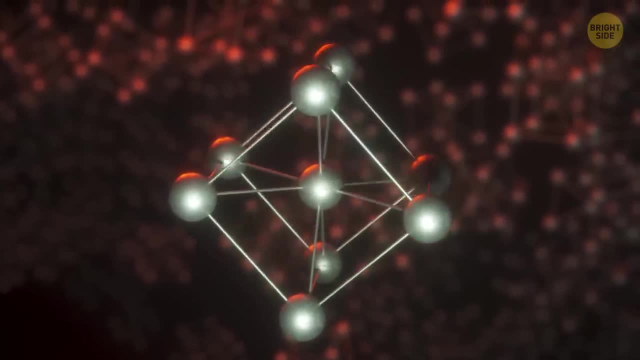 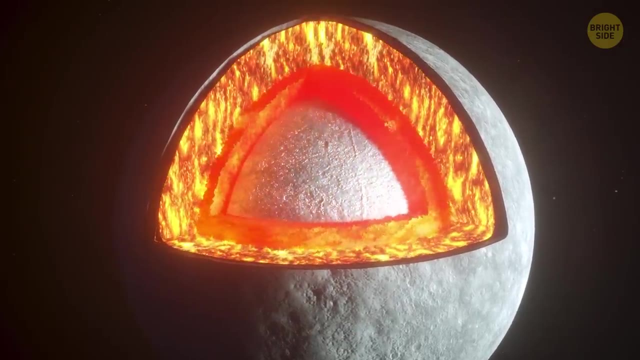 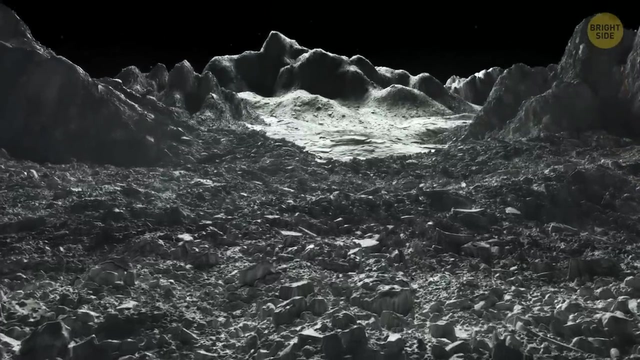 Its core contains more iron than any other planet of the solar system. Recently it's been discovered Mercury might have a solid inner core along with its outer core that consists of liquid metal. The planet's outer shell is composed of a rocky mantle and solid crust which is just 250 miles thick. 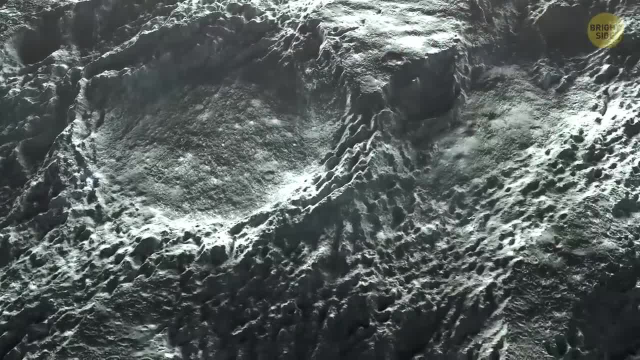 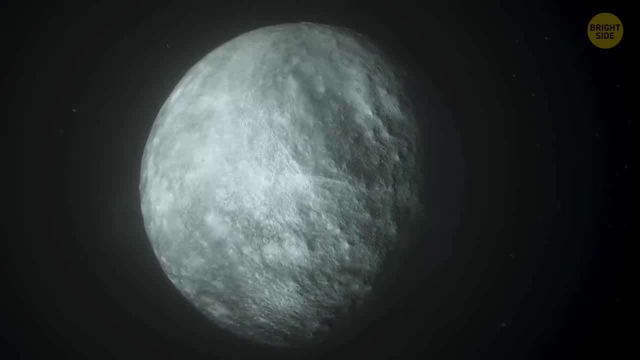 Mercury is too small to hold on to its atmosphere made up of hydrogen and helium. The planet is also too close to the Sun. That's why the solar winds keep sweeping away the little atmosphere the planet manages to gather. Whoops, there it goes. 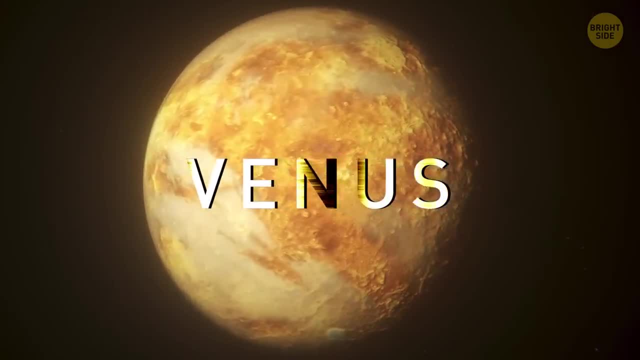 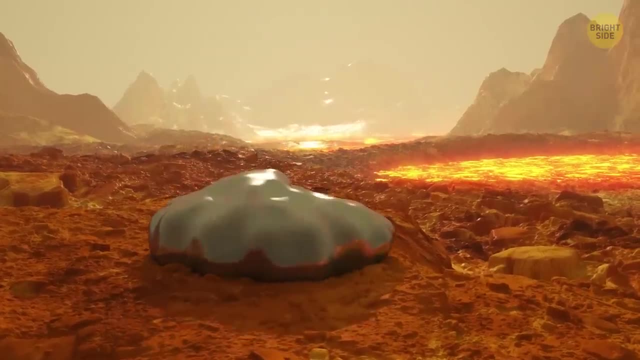 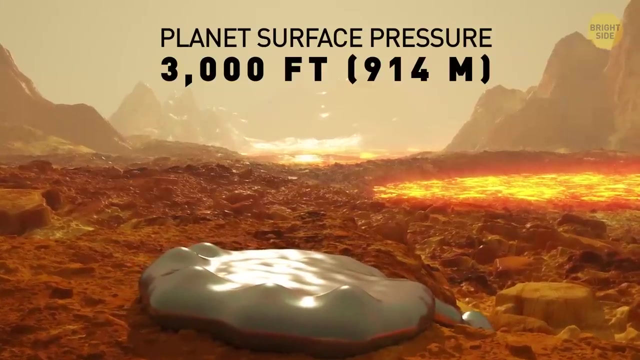 Venus, Our next stop, is the hottest planet in the solar system, with average temperatures reaching 870 degrees Fahrenheit. It means lead would melt if you brought it to Venus. The pressure on the planet's surface is the same as at a depth of 3,000 feet underwater on Earth. 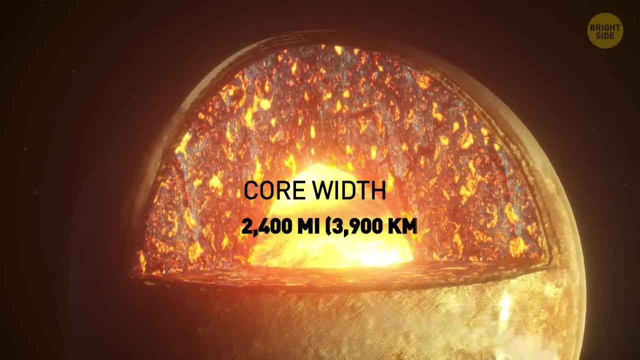 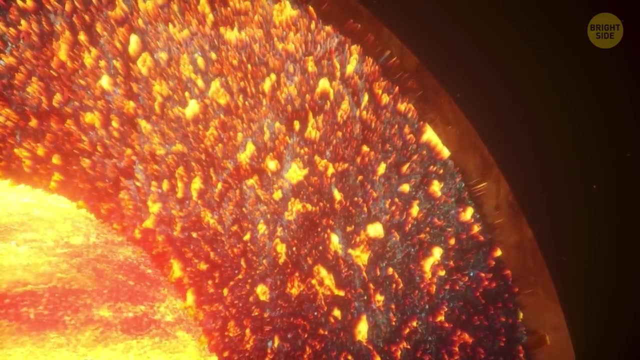 The planet's metallic iron core is 2,400 miles wide, which is almost as the distance from New York to Los Angeles. The next layer is a molten rocky mantle that's 1,200 miles thick. Venus' insides are covered with a crust. 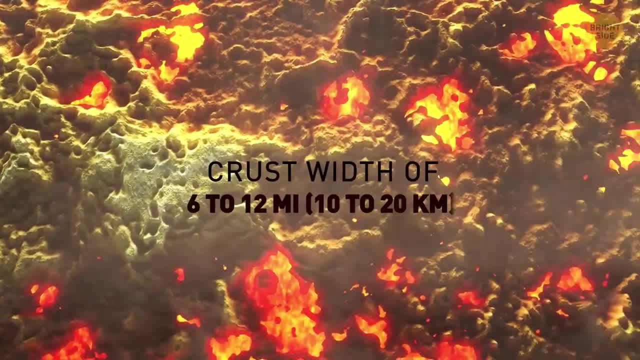 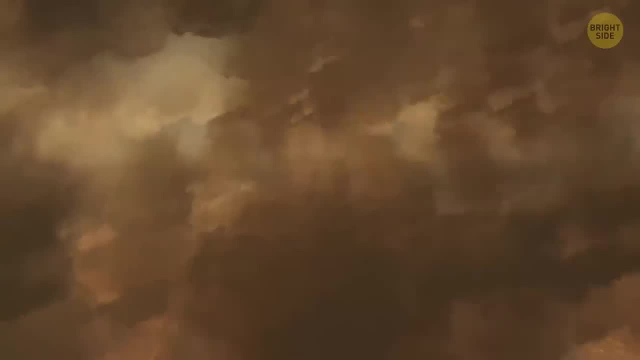 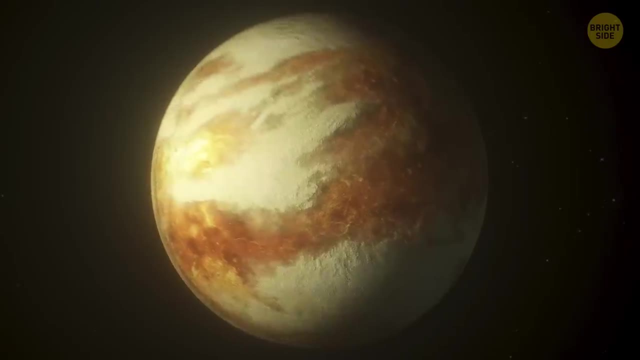 It consists mostly of basalt and is 6 to 12 miles wide. The planet's thick atmosphere is nightmarish: It's 96% of carbon dioxide, with 3% of nitrogen and thick clouds of sulfuric acid. Venus also has a heck of a serve. Her sister, Serena, is even better. Oops, wrong Venus, never mind. 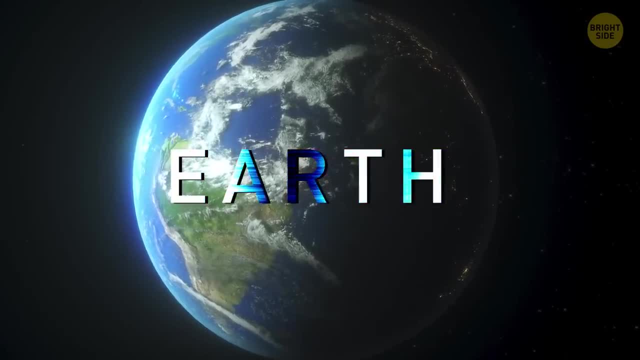 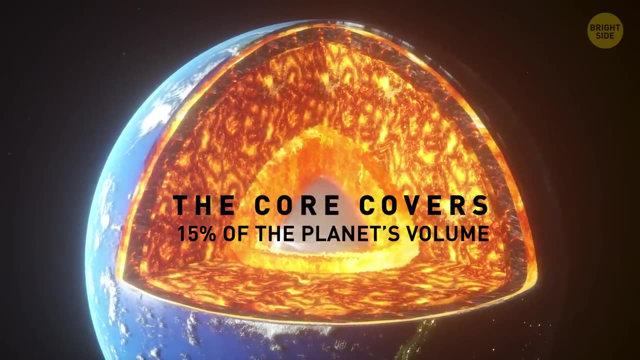 Earth. We've reached our home planet, the densest in the solar system. At the Earth's center there's a core that takes up 15% of the planet's volume. It consists of two parts: the outer and the inner core. 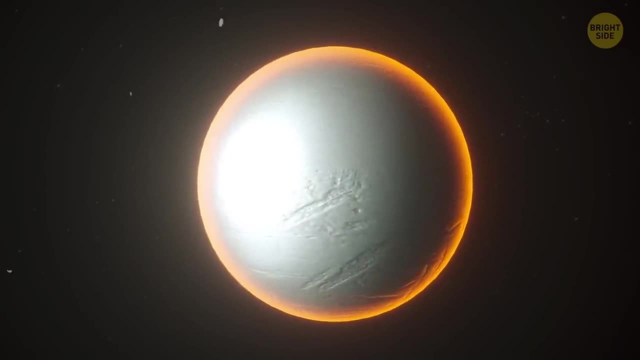 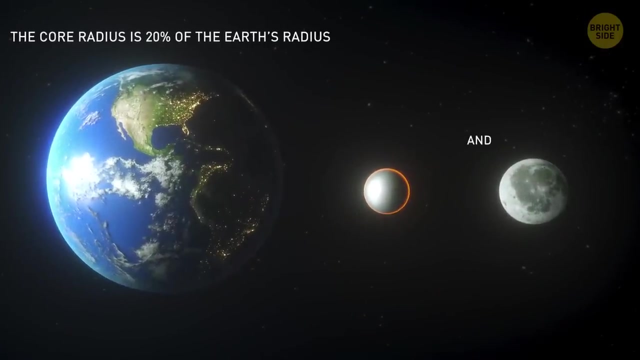 The inner core is a solid ball made of iron and nickel. Its radius is 760 miles give or take, which makes 20% of the entire Earth's radius and 80% of the moon's radius. The 1,500 mile thick outer core is liquid. 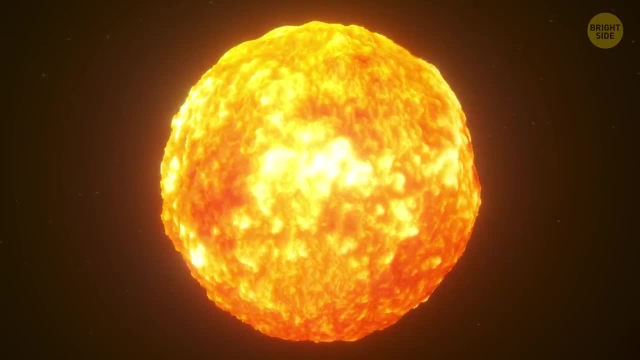 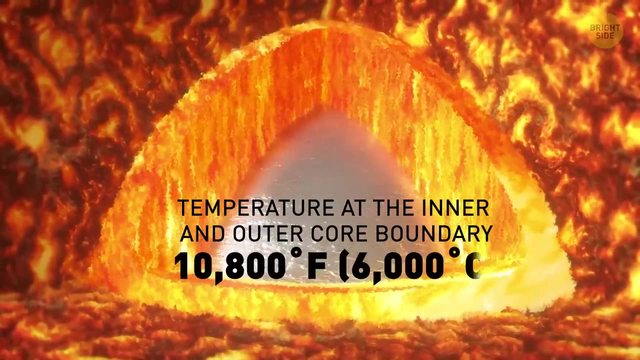 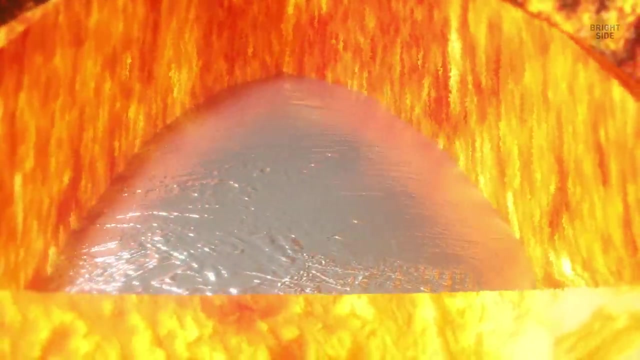 It also consists of iron and nickel, but it's not under enough pressure to be solid. The temperature at the boundary of our planet's inner and outer core is 10,800 degrees. That's as hot as the surface of the Sun, And the pressure there is three and a third million times the atmospheric pressure at sea level. 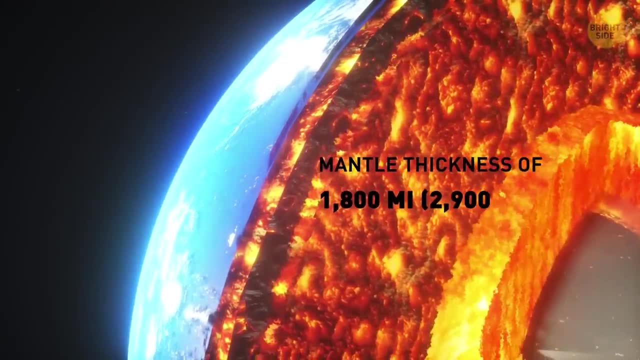 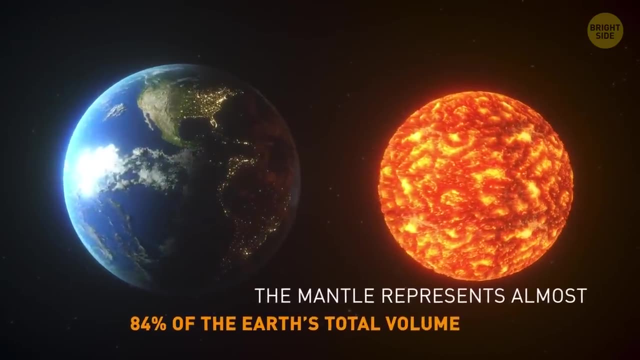 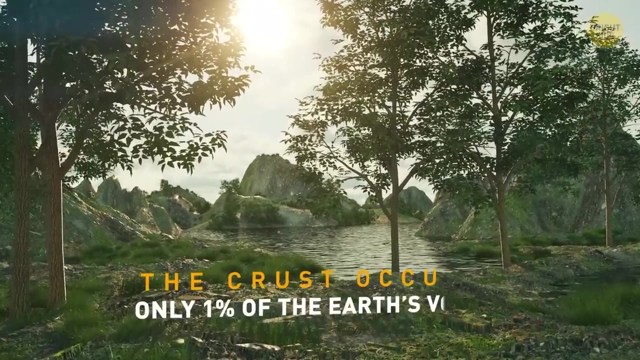 The mantle surrounds the outer core. This layer is about 1,800 miles thick and makes nearly 84% of the entire Earth's volume. It consists of silicate rocks rich in iron and magnesium. The crust is a relatively thin layer that takes up only 1% of the Earth's volume. 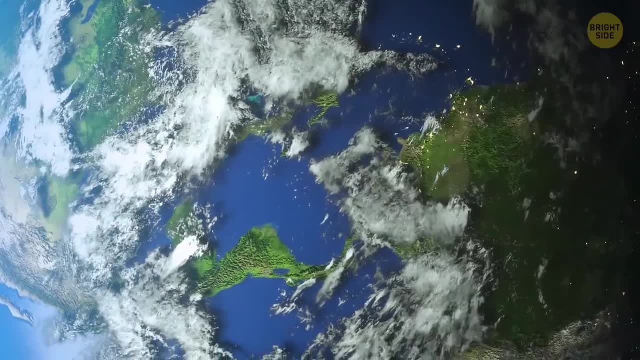 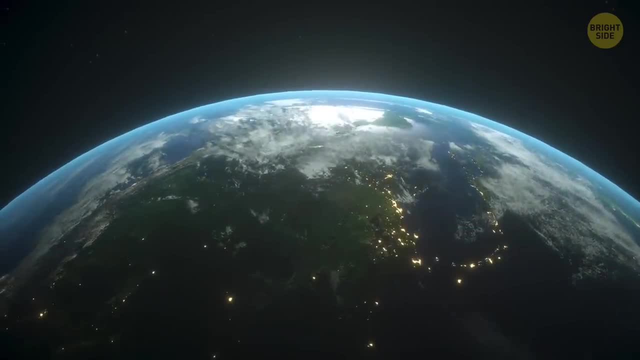 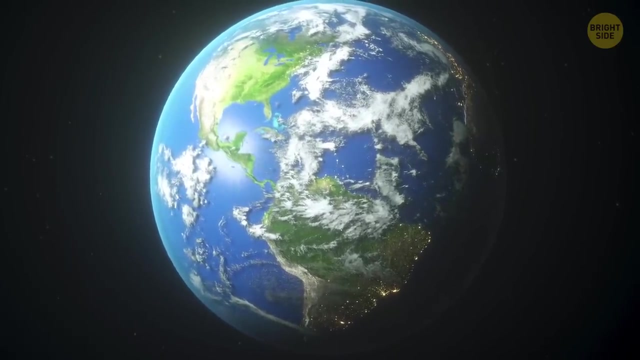 Hey, I like thin crust Along with the upper part of the mantle. it's broken into tectonic plates. They move as fast as your fingernails grow and let heat escape from the Earth's interior. The crust is mostly made up of oxygen, silicon, aluminum, iron and other minerals. 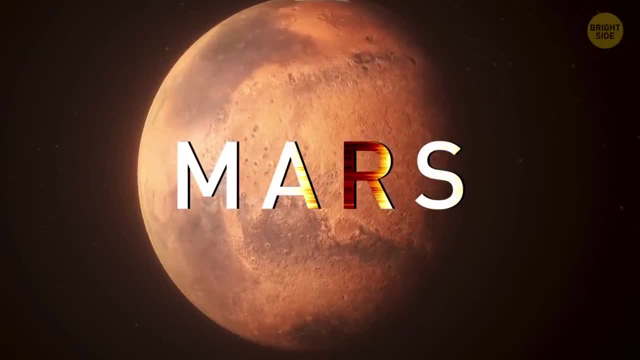 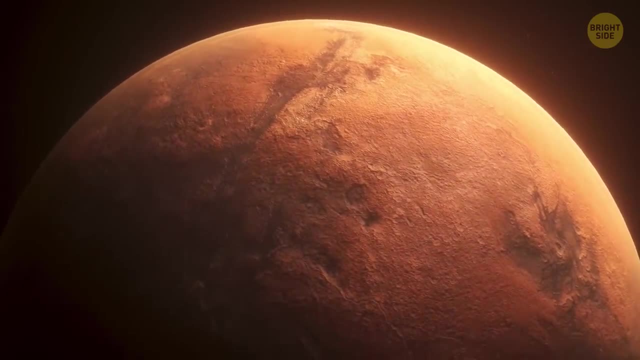 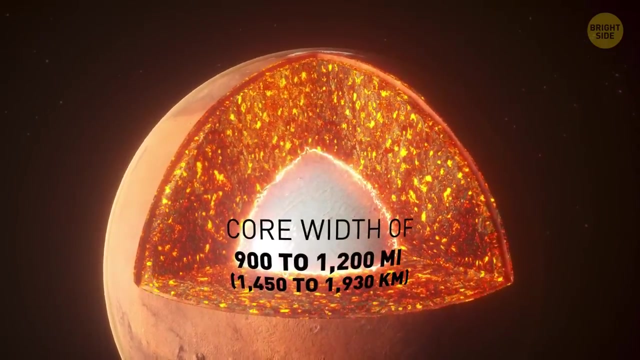 Mars, But it's time we leave our planet behind and move to the red planet. It's the last of the inner planets, which are also called terrestrial, since they're made up of rock and minerals. Mars has a core made mostly of iron, nickel and sulfur. It's between 900 and 1,200 miles across. 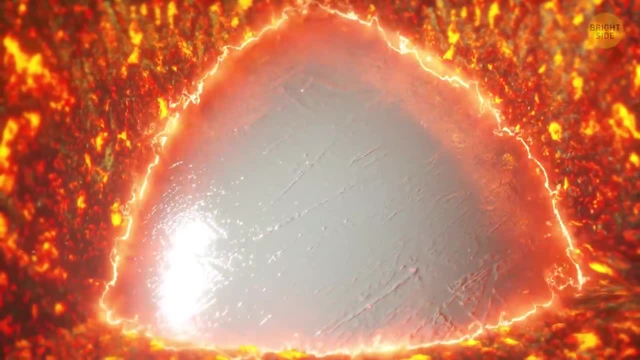 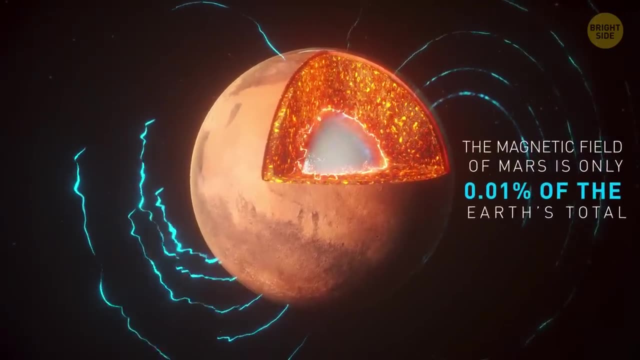 The core doesn't move. That's why Mars lacks a planet-wide magnetic field. The weak magnetic field it has is just 0.01% of the Earth's. The mantle surrounding the core is composed of thick silicates, oxygen and some other minerals. 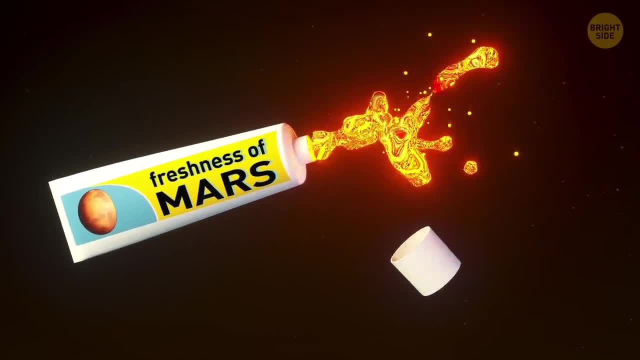 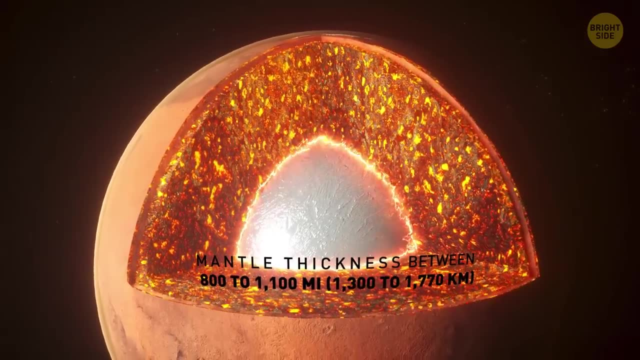 You can probably compare it with soft, rocky toothpaste. Yeah, brush your teeth with that. The Mars mantle is also much thinner than the Earth's: It's just 800 to 1,100 miles thick. The planet's thin crust consists of volcanic basalt rock. 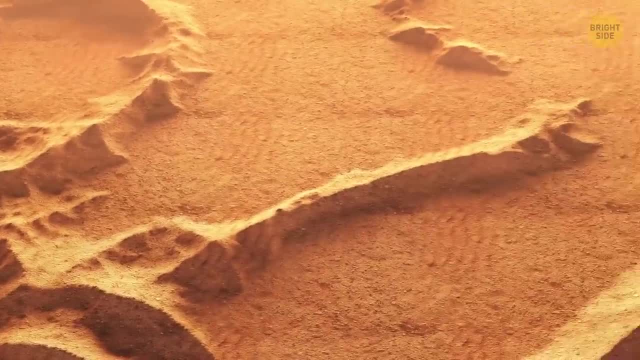 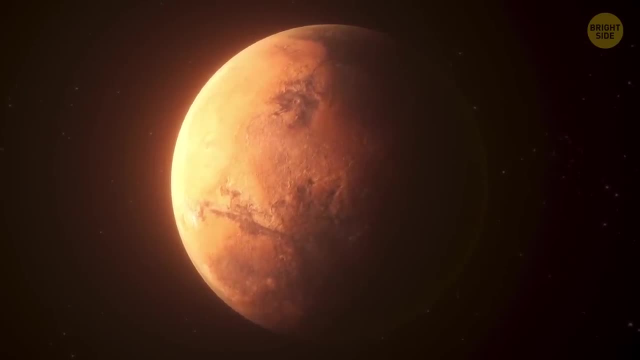 Astronomers believe it isn't broken into tectonic plates and remains in one piece. The crust is covered with fine reddish rock. The crust is covered with fine reddish dust that looks like talcum powder. I like my crust covered with tomato sauce and cheese. 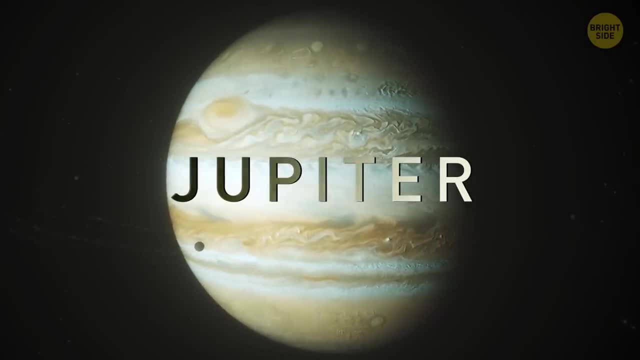 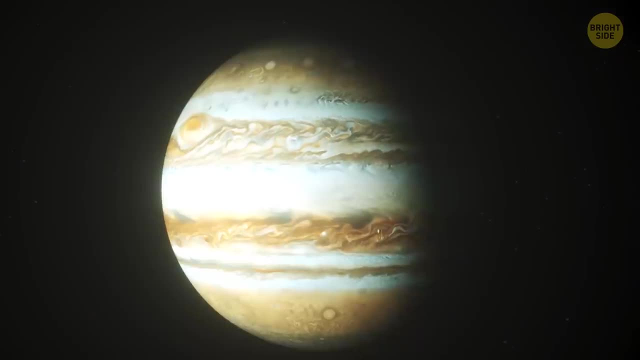 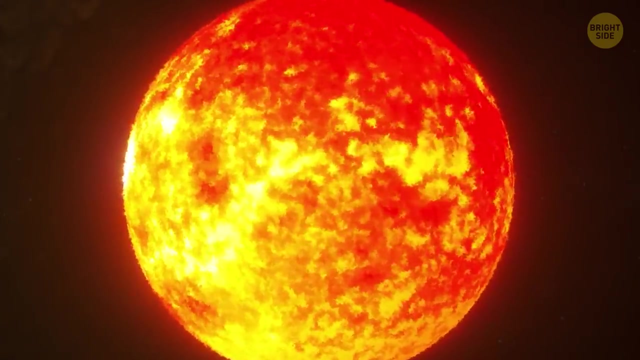 Jupiter, The next planet on our way, is very different from the ones we've already visited. The largest planet in our solar system, Jupiter, is a gas giant. If the planet was 80 times as massive as it is now, it would have a chance to turn into a tiny red dwarf star. 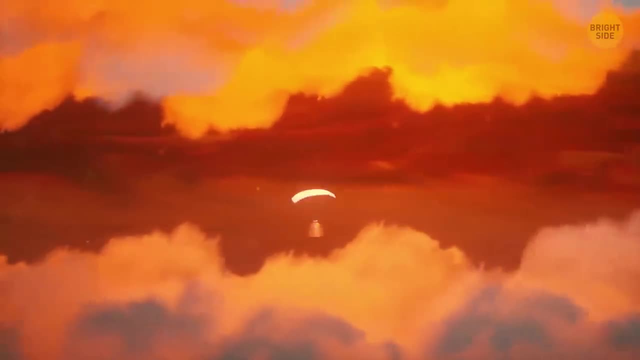 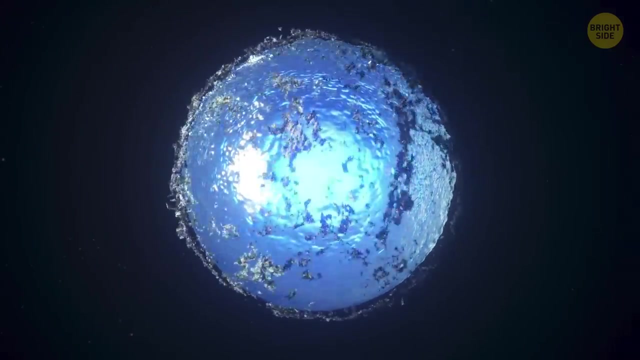 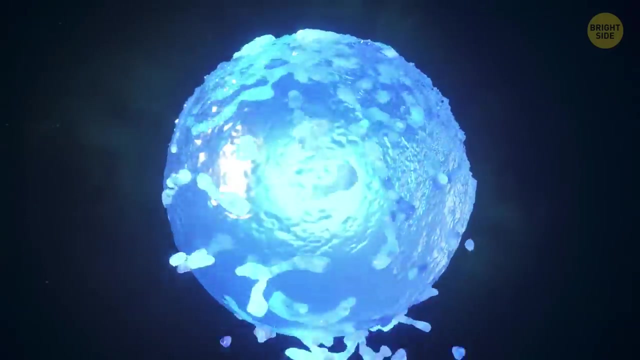 Anyway, if you decided to parachute into Jupiter, you would never land on a firm surface. It's still unclear whether the planet's core is a molten ball of liquid or a solid rock 14 to 18 times the mass of Earth. There's even some evidence the gas giant's core might be melting right at this moment. 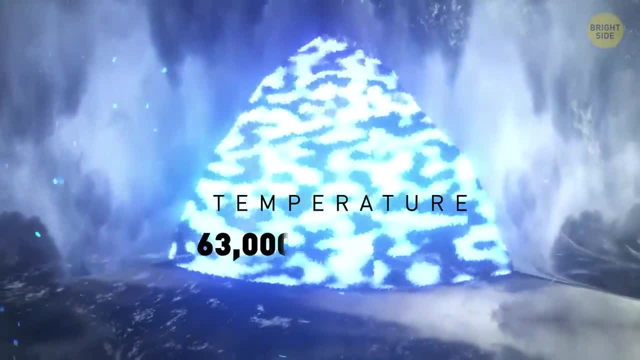 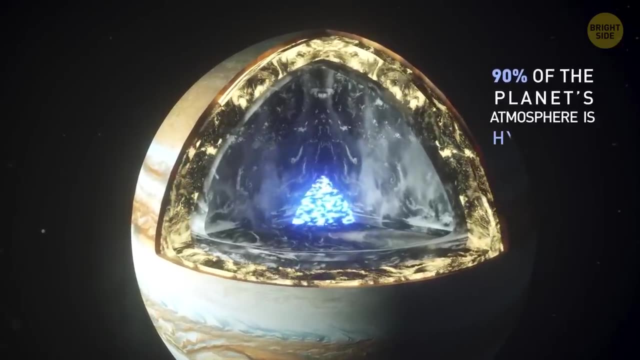 Whatever the truth is, the temperatures at the center of Jupiter reach 63,000 degrees, give or take. Around 90% of the planet's atmosphere is hydrogen. The remaining 10% is made up of helium with tiny traces of oxygen. Under immense atmospheric pressure, hydrogen and helium gases turn into a dense fluid. the deeper you go, Closer to the core, this liquid becomes the mixture of metallic hydrogen and helium. There's no solid ground on the planet. That's why astronomers define the planet's surface as the point where the atmospheric pressure equals that on Earth. 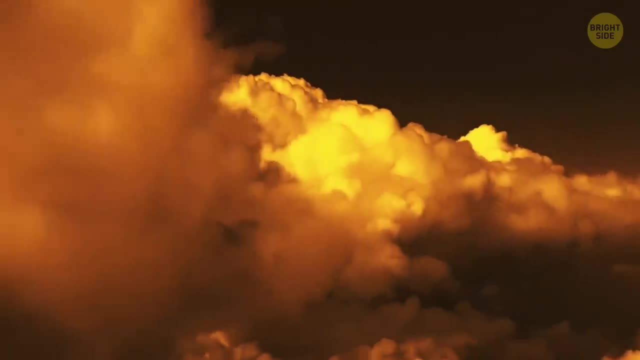 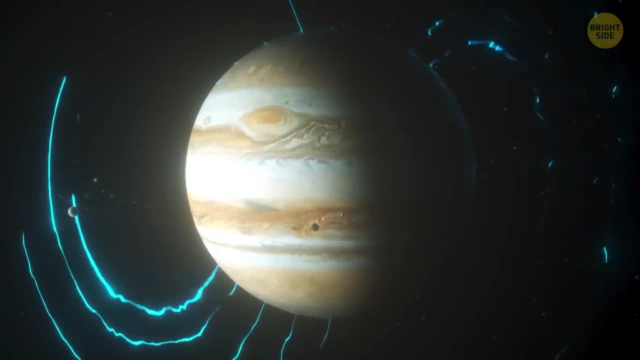 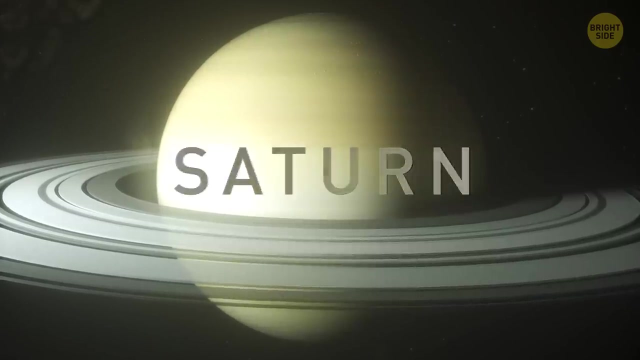 You wouldn't be able to stand on that surface, though It's just another layer of gases, But the gravitational pull there is more than 2.5 times more powerful than that on our planet, Saturn. Welcome to the planet with the winds that travel at more than 1,100 miles per hour at the equator. 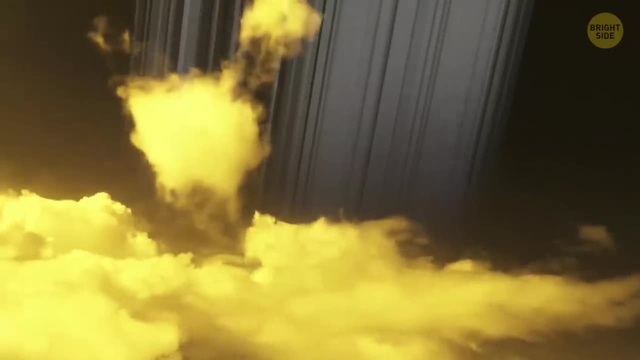 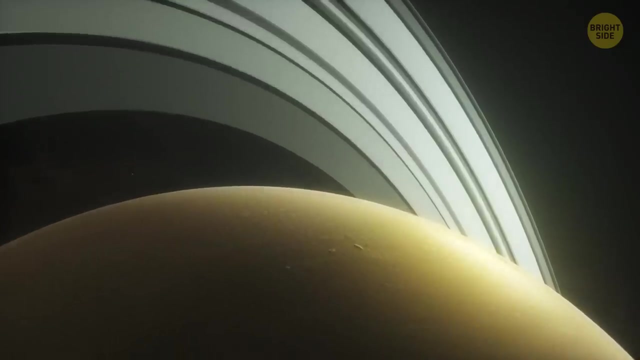 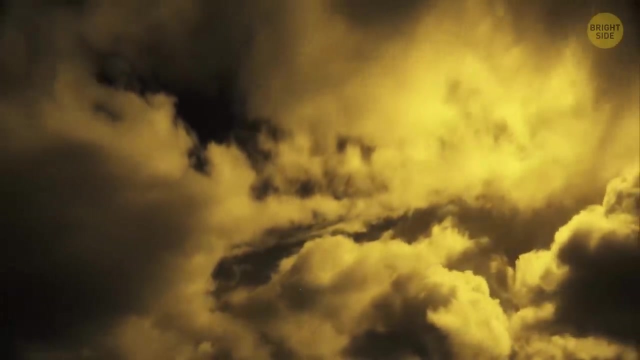 It's also the planet with the big rings. Saturn is mostly composed of hydrogen and helium, with some traces of methane, ammonia and water, But it contains more sulfur than Jupiter, which gives the planet a smog-like orange hue. The atmosphere of Saturn isn't really different from its surface. 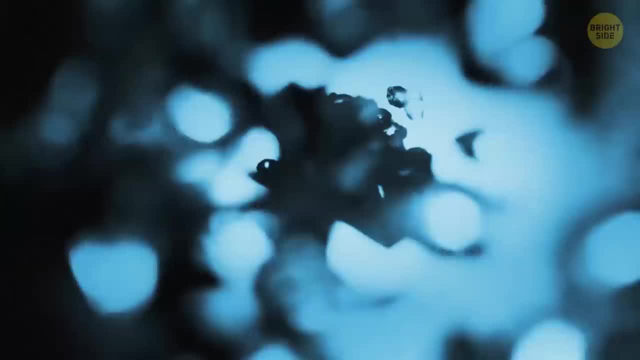 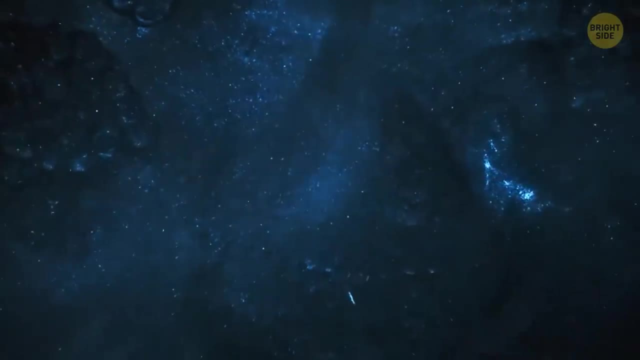 But the deeper you go, the higher the pressure becomes and hydrogen becomes liquid. Further to the center of the planet, this liquefied gas turns into metallic hydrogen. Like Jupiter, Saturn might have a rocky core with hydrogen and helium surrounding it. 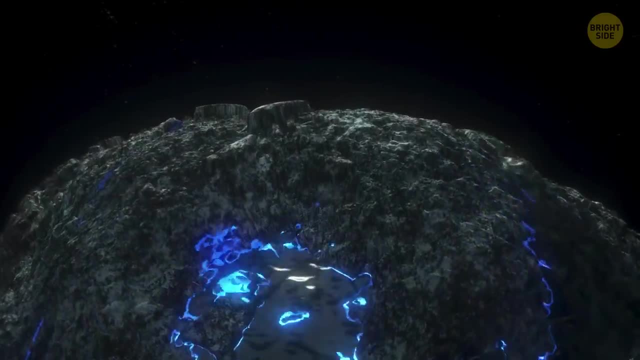 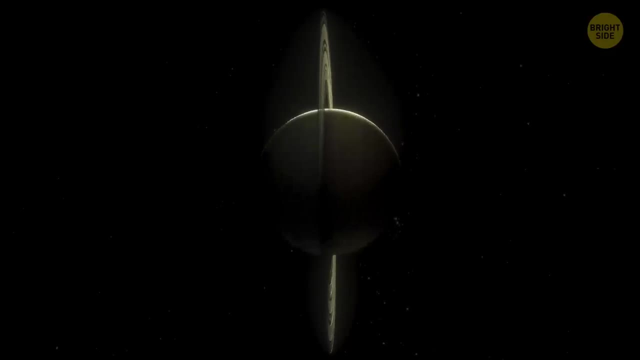 On the other hand, even if it's made up of rocky material, the core can still be liquid. Saturn is the least dense planet in the solar system. It has one-eighth the average Earth's density. The planet is 95 times more massive than Earth. 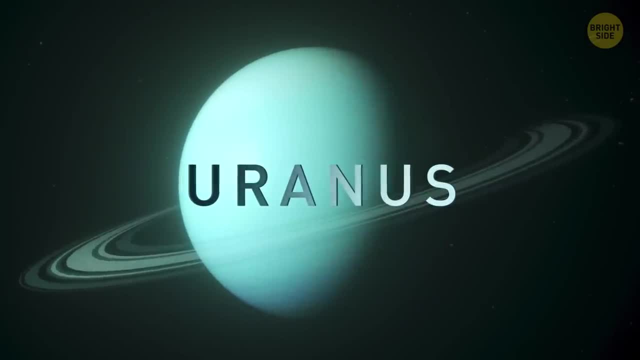 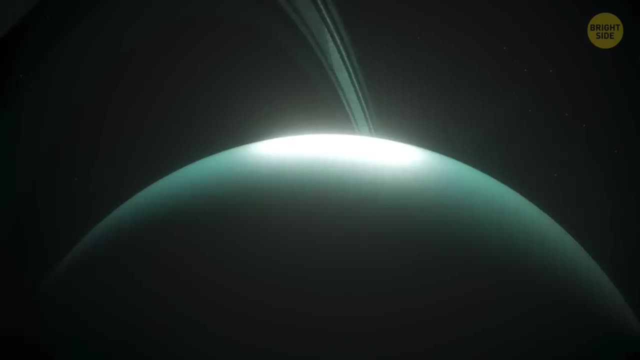 Uranus. Look at this blue-green planet on our way. It's one of the two ice giants in our solar system. It's composed of more ice than gas. At the very center of Uranus there is a rocky core small just half the Earth's mass. 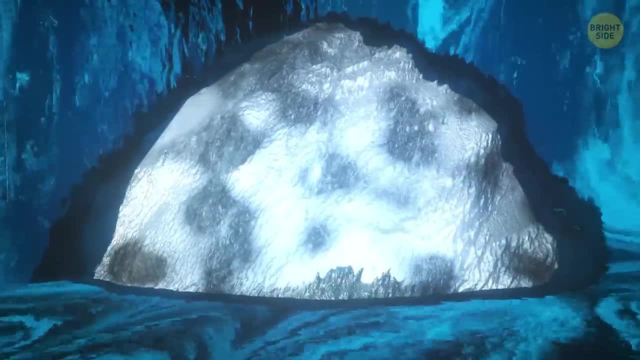 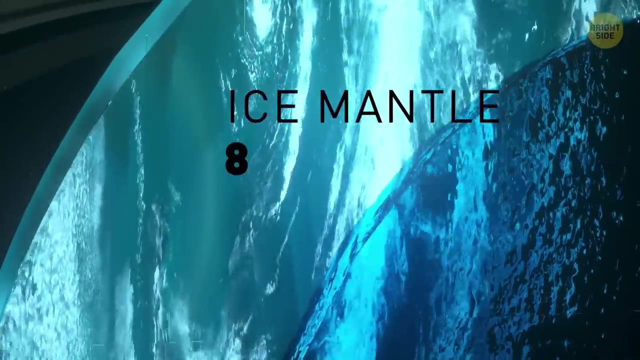 Compared to other planets, Uranus' core is rather cool. Only 9,000 degrees An ice mantle surrounds the solid core and that's the largest portion of the planet- about 80%. It's also not the ice you might be thinking about. 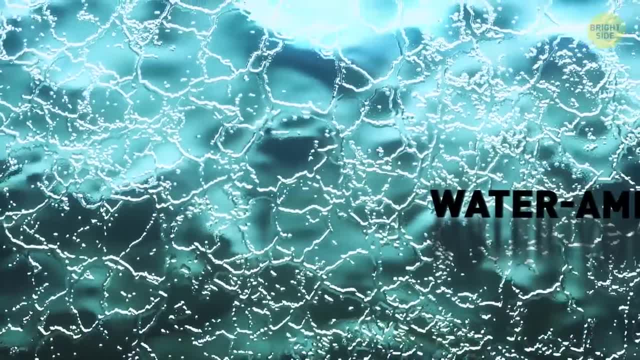 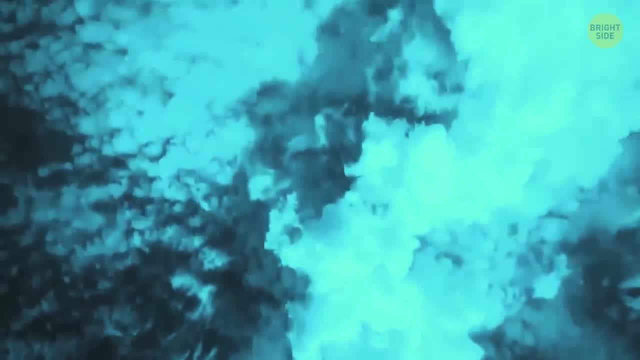 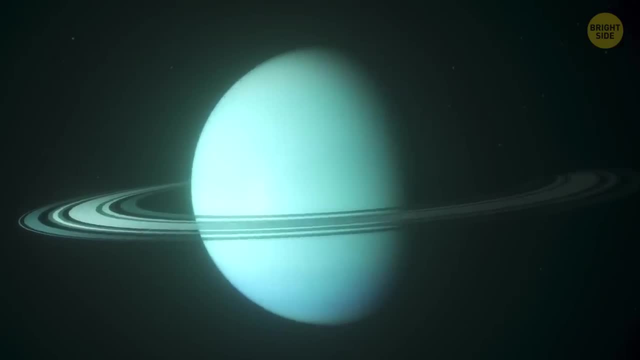 It's a hot, dense fluid made up of water, ammonia, ice and methane, sometimes referred to as a water-ammonia ocean. Uranus' atmosphere is mostly hydrogen and helium, But it has its blue-green color because of methane, gas that absorbs the red light. 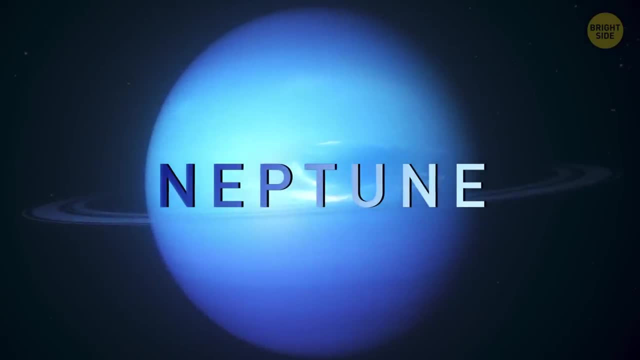 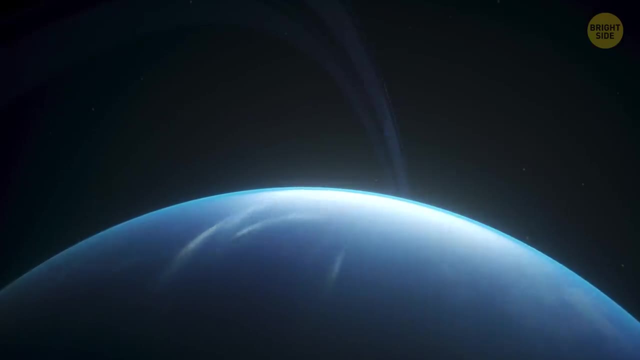 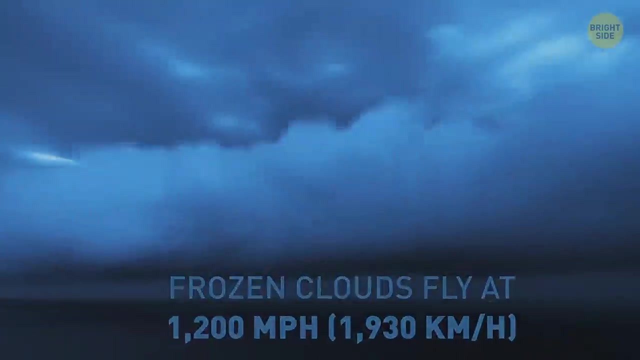 Neptune. That's the final stop of our unusual journey and the second of the two outer planets known as ice giants. It's also the windiest place in the solar system. Clouds of frozen methane are whipped across the planet at a speed of 1,200 mph.